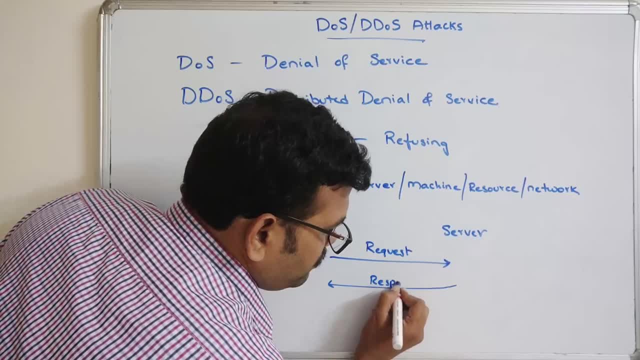 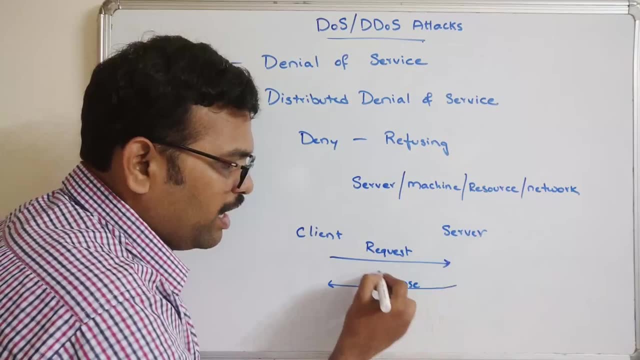 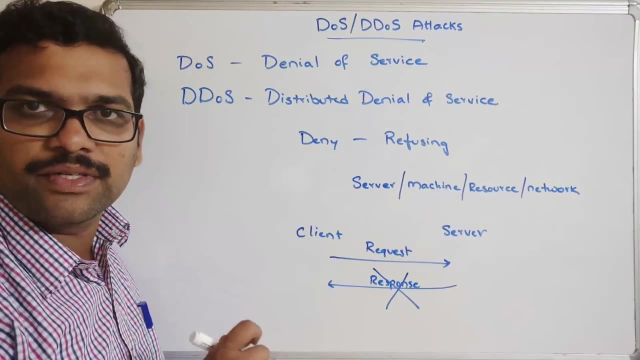 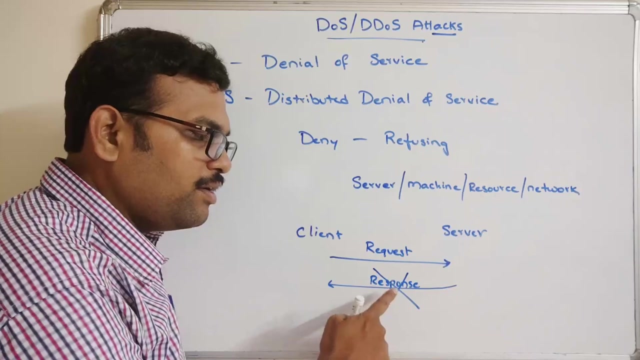 the server will send the response. So that means the server is giving some sort of service to the client. And if the server refused his response to the client, that implies denying of service, Then why we are calling it as an attack? So this deny is done by the attacker, right? So the attacker? 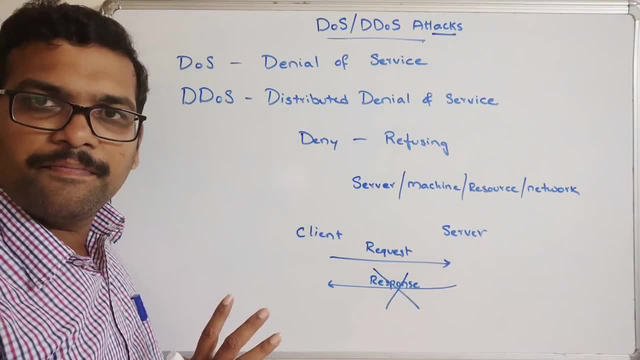 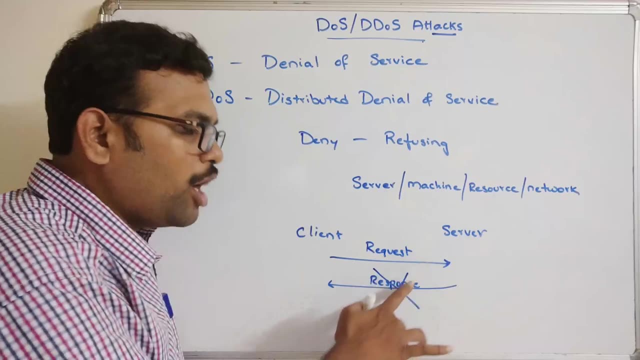 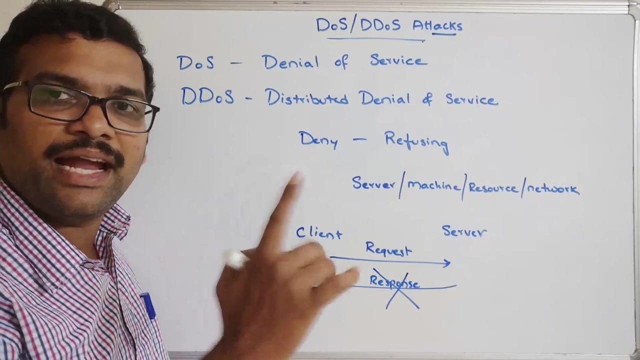 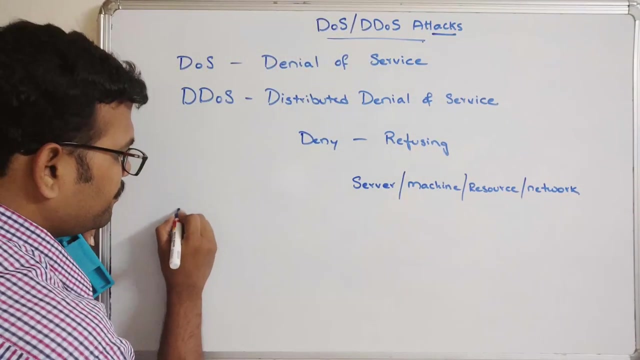 makes the server to refuse the response to the client. Okay, so the attacker will make the server down and stops the service to the, its clients, to its clients, So that we call it as a denial of service. is attack right? so I'll write an exam. I mean definition here. so this attack dos attack. so 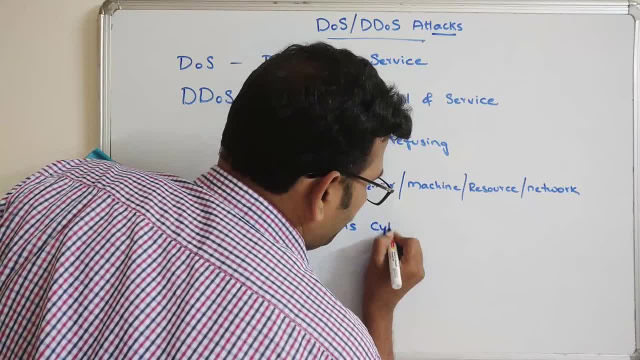 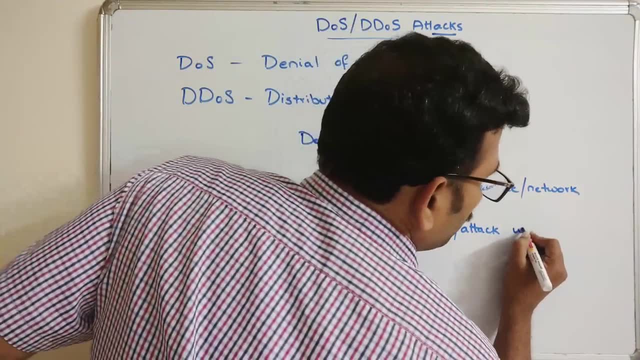 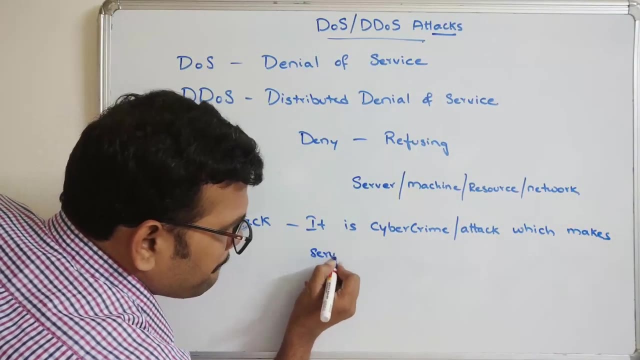 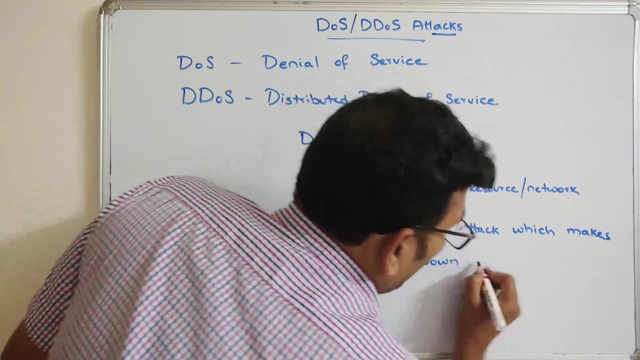 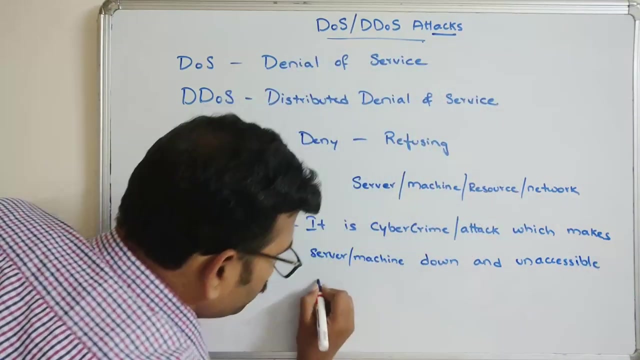 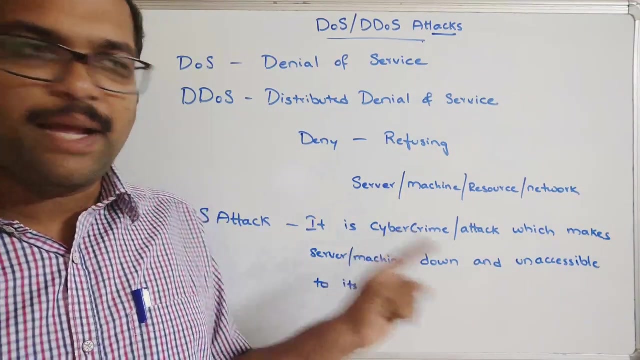 it is a cyber crime. it is a cyber crime or an attack or an attack which makes the server or a machine, which makes a server or machine or any other resource down and unaccessible so it can't be accessible, right accessible to its users. it's called DD voice attack. so it is a cyber crime, or 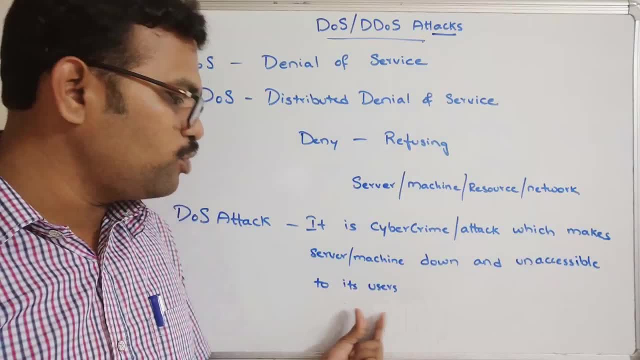 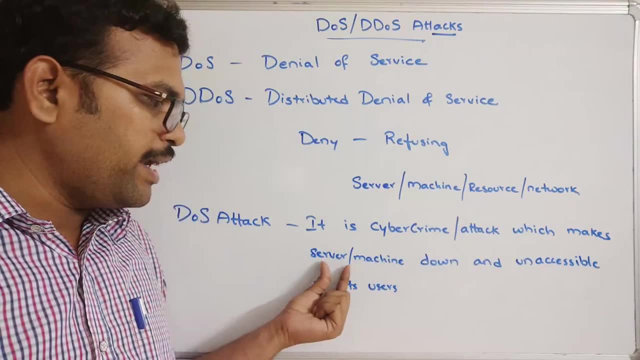 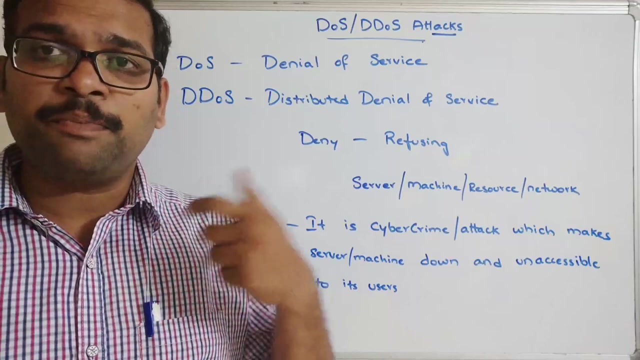 attack which makes the server down and unaccessible to its users. so how the attacker will make the server down, okay, how the attacker makes a server down, obviously, if the server is down it can't be accessible, so that implies it can't respond to all this. all the services, I mean all the requests- are coming from its claims. so 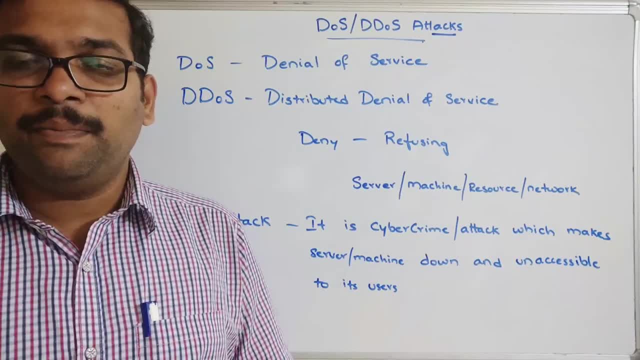 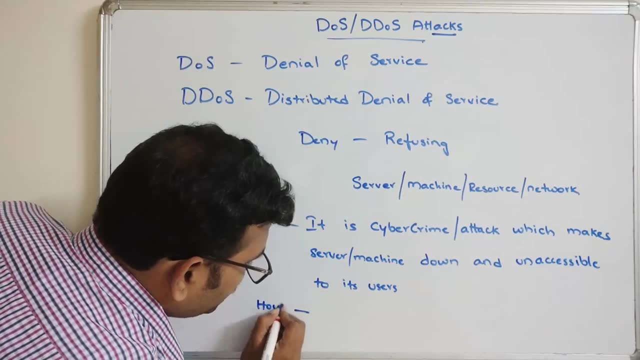 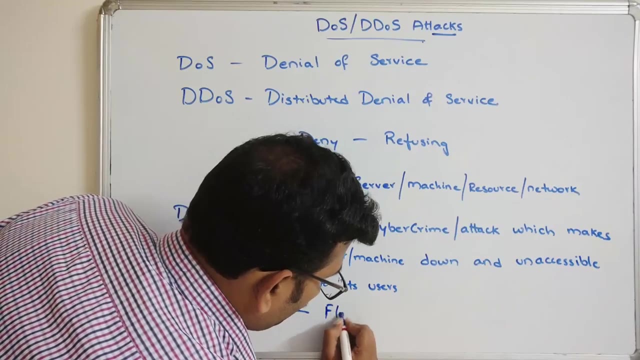 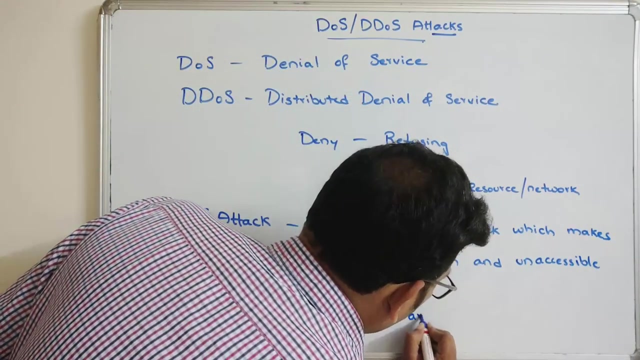 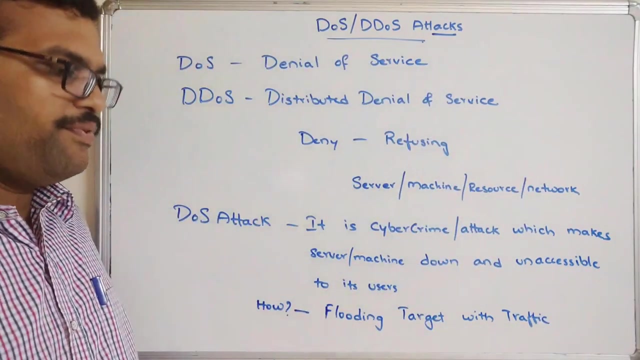 obviously the server will refuse the request. that means they will the service. so how? so how these attacks will done, how this attack will done. so the attacker will do the attack by flooding target with a traffic flooding. the target with the traffic flooding means more number of requests. 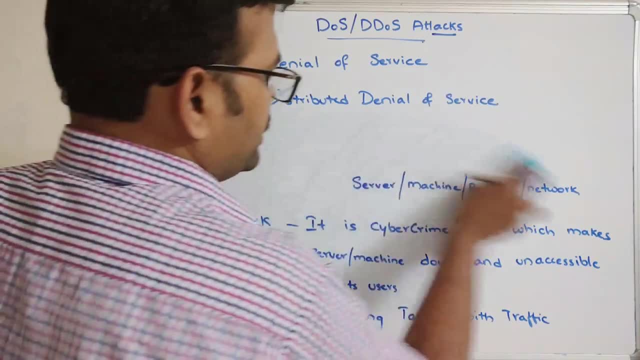 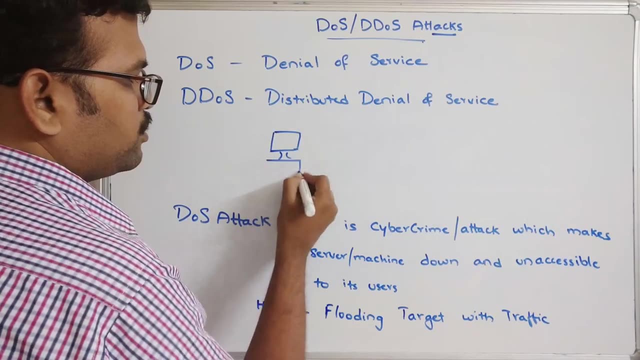 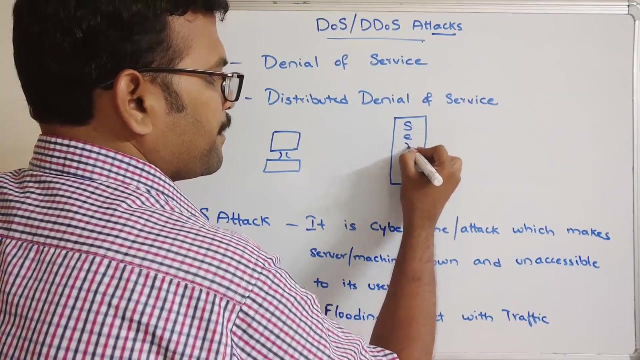 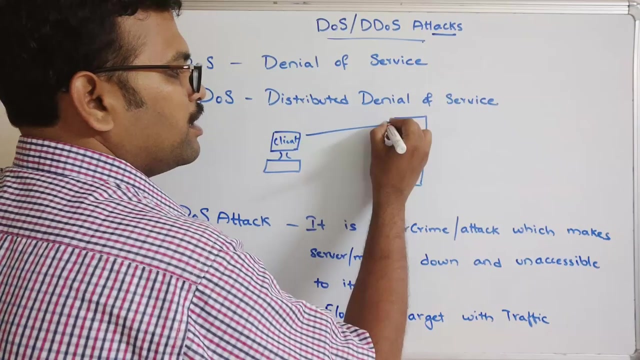 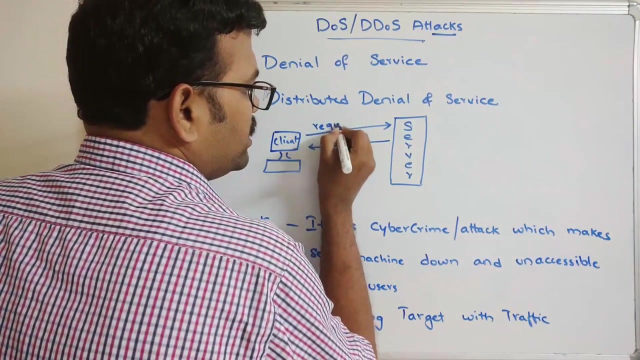 resending the request. okay, let us let me explain the with an example. so let us take one client as a server, so this is a client, and let it be. this is a server, so this is a client. so obviously a client will send the request and comes the response. okay, so it is a request and it is a response. 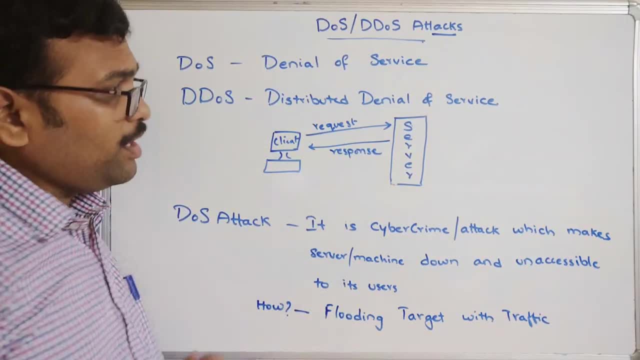 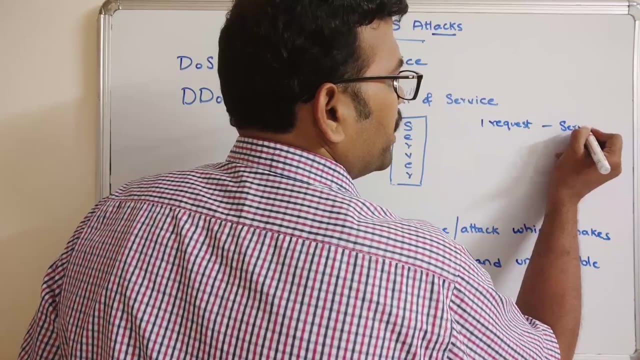 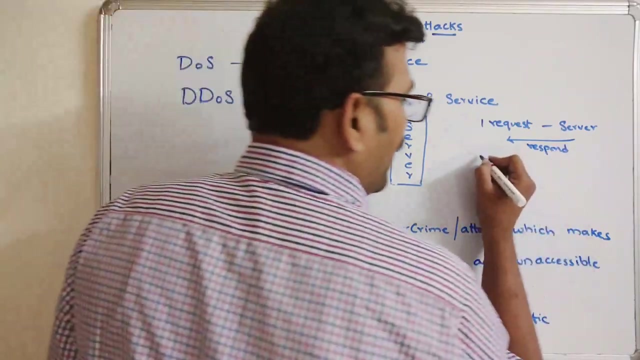 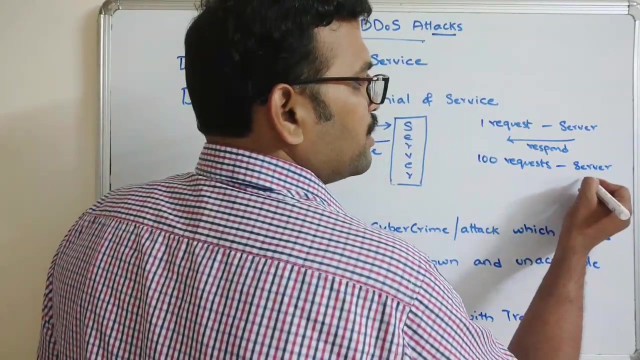 So everything will be fine, Right? So if one request, if one request is sent to server, automatically the server can respond. The server can respond, Right? If 100 requests, if 100 requests were sent to a server, obviously the response will be slow. 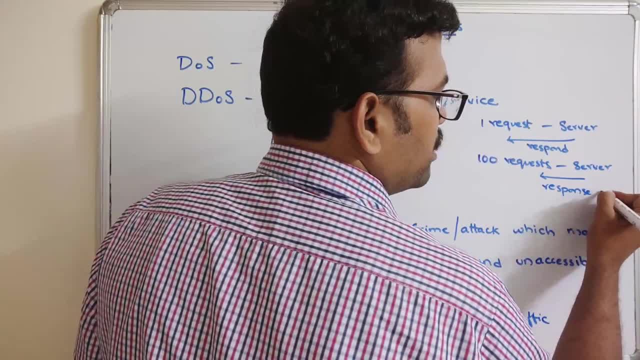 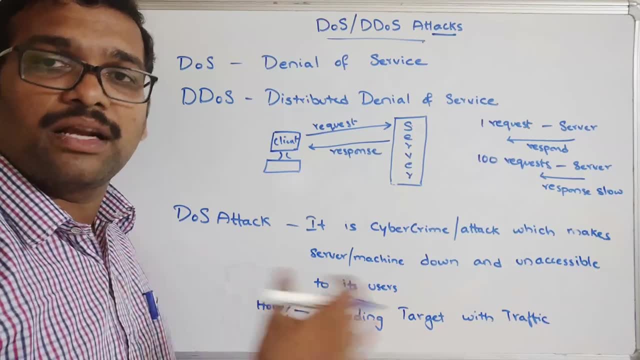 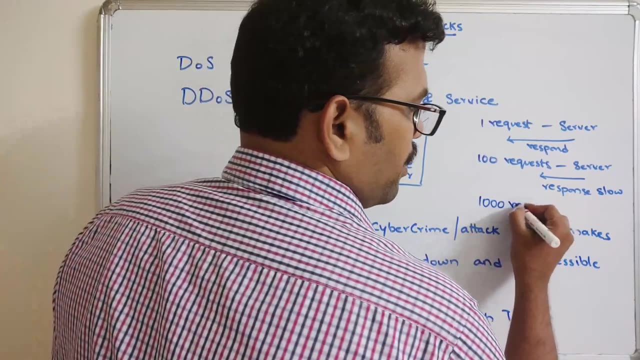 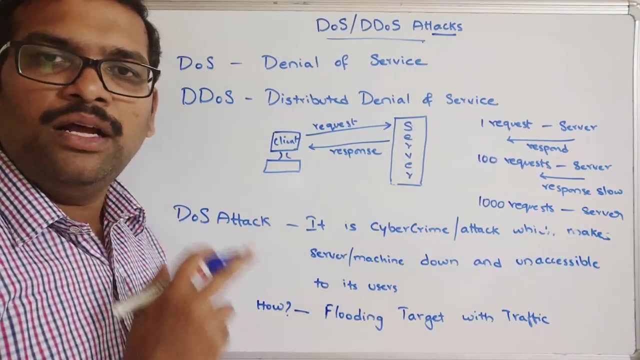 The response will be slow. That means there will be some sort of delay in the response because the server has to give the service for all the requests And if the same thing happens for 1000 requests, if the same thing happens for the 1000 requests, so obviously the server can't respond to all the requests, So obviously it can't be accessible. 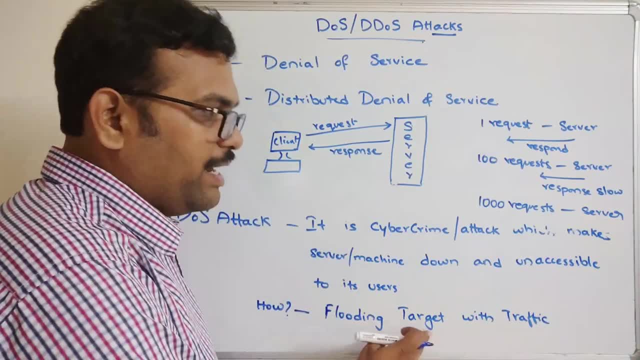 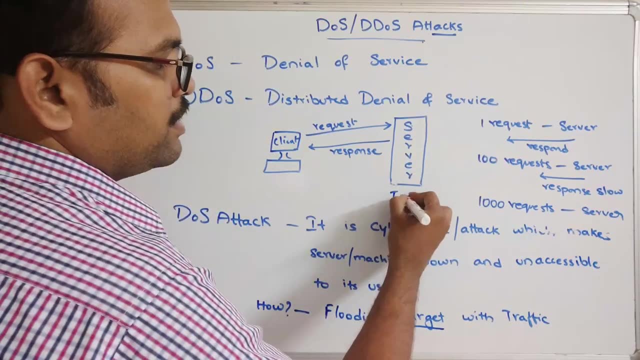 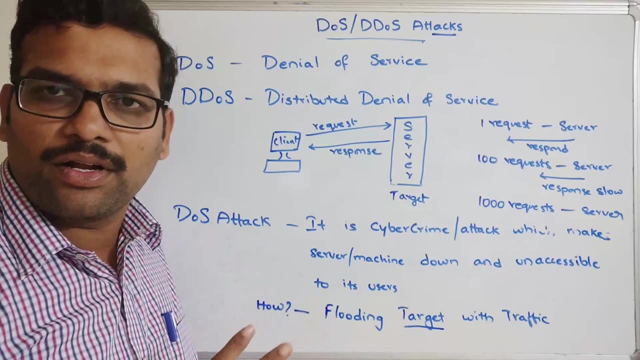 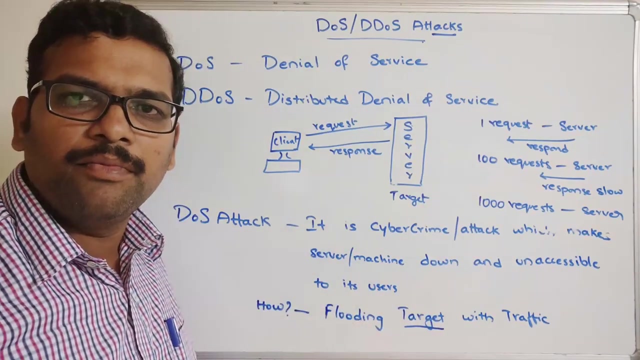 So So the attacker will flood the target, flood the target with the traffic. So what is this target? So here the target will be the server. Target will be the server, or any machine or any resource or any network, whatever it may be. So the attacker will flood the target with a more number of traffic. So, for example, consider the client and server. So a number of traffic. 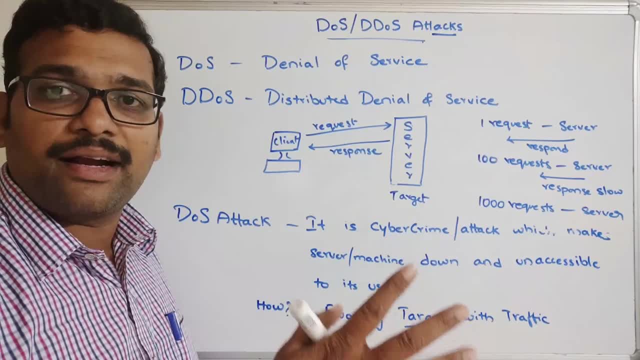 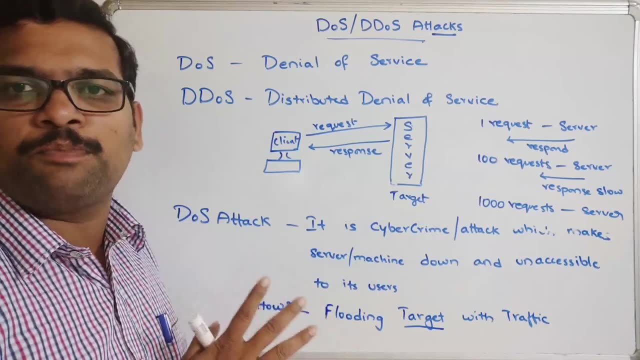 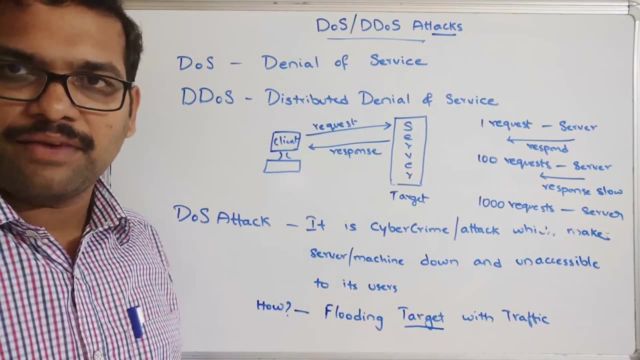 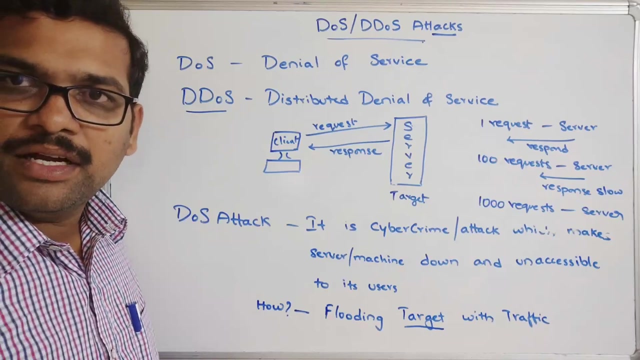 So a number of requests will be sent from the client to server so that the server can't respond to each and every request coming from the client. That implies so that server is refusing to respond and it is unaccessible, Right? So such type of attacks, we call it as a denial of service. Denial of service. And then what is this? DDoS? Distributed denial of service. Distributed denial of service, For example. 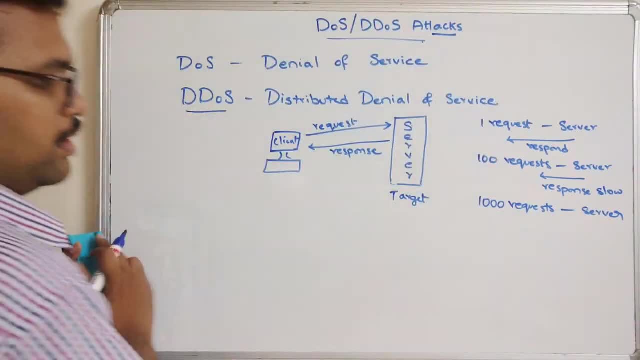 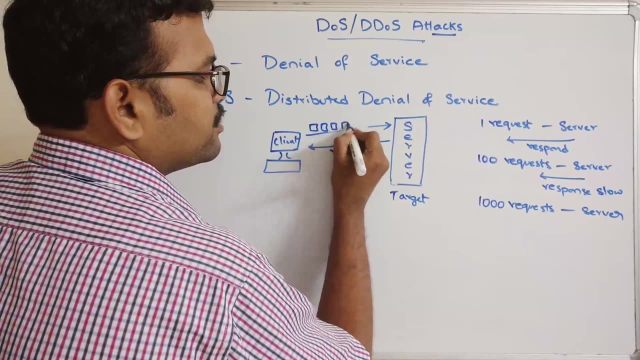 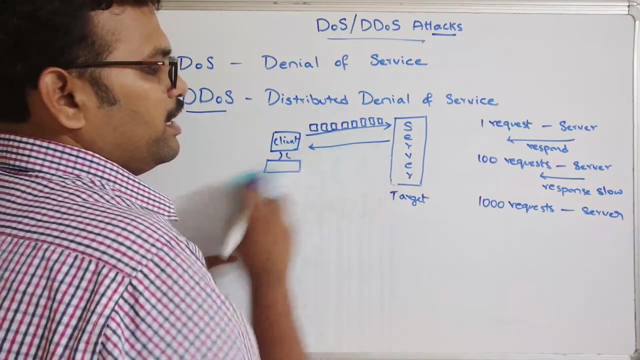 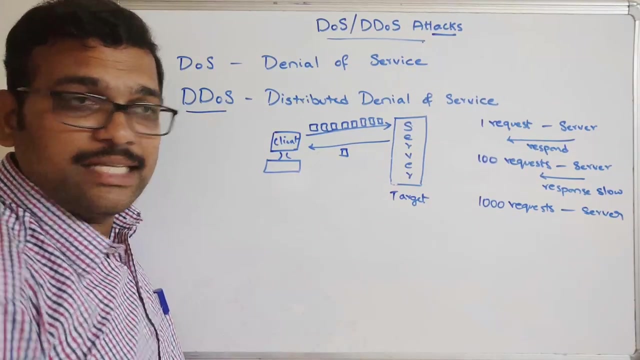 See here, if the client was sending continuously the packets, so thousands of packets, thousands of requests to the server. so obviously it can't respond to all the requests from the client coming from the client, Right? So in such a way the server will refuse the request coming from the client And similarly. 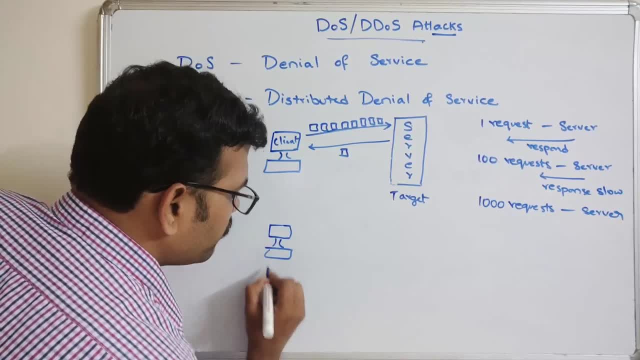 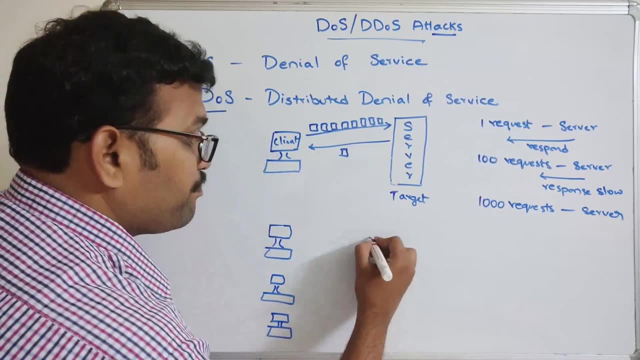 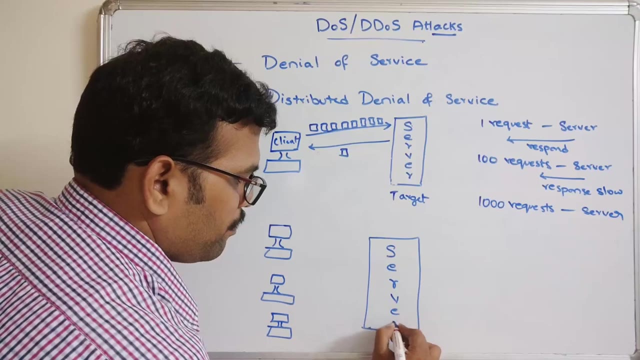 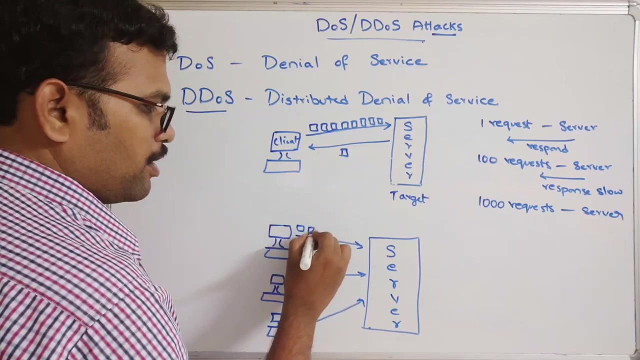 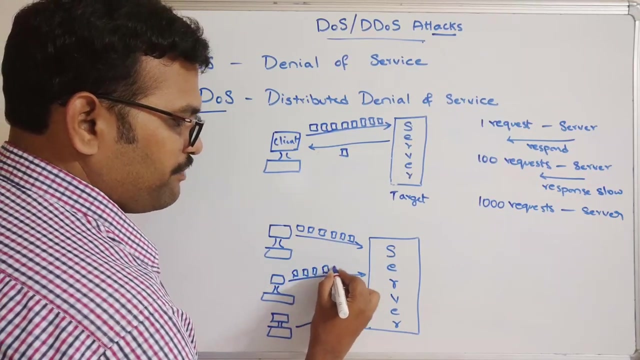 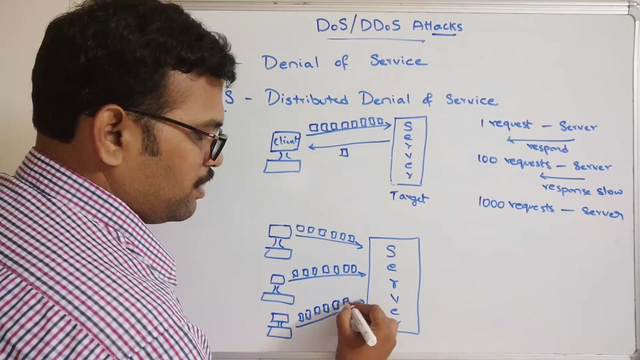 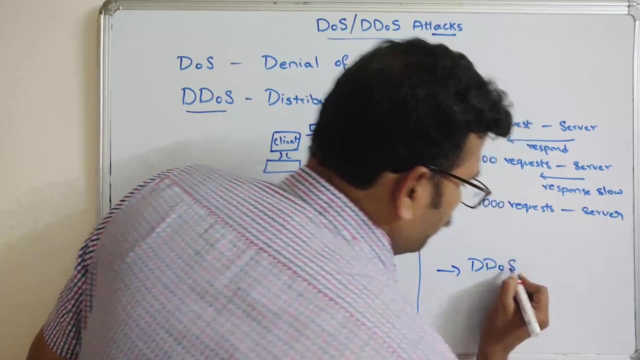 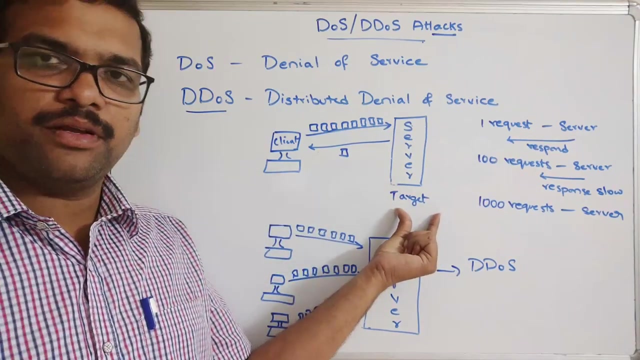 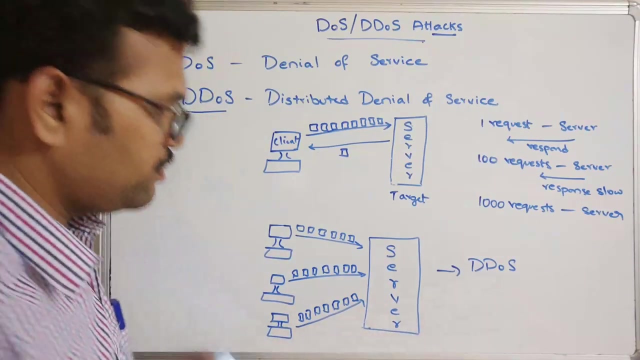 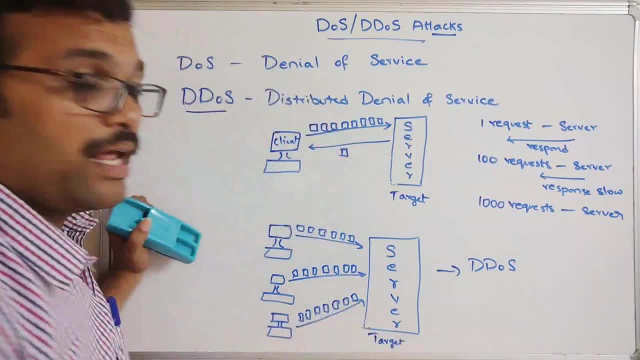 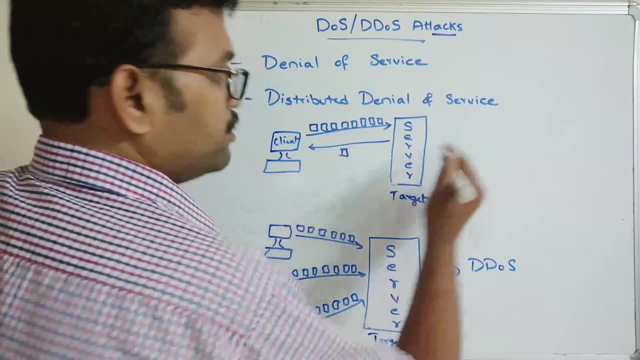 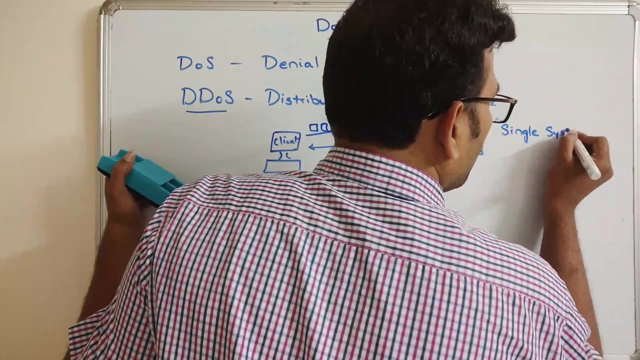 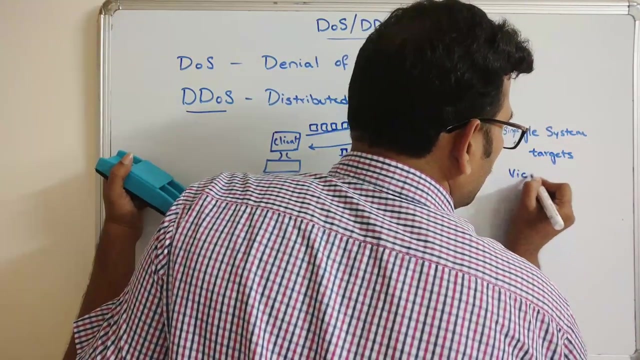 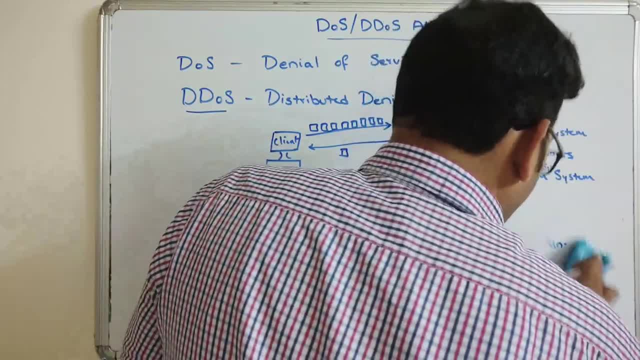 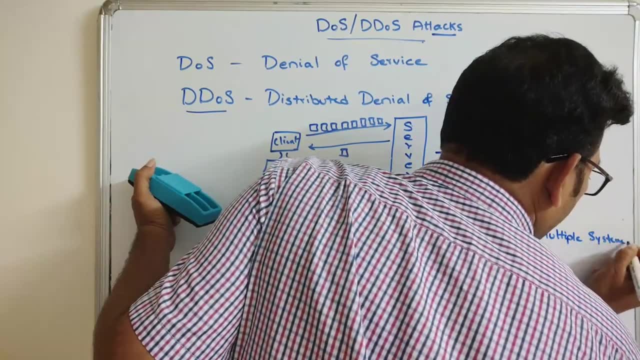 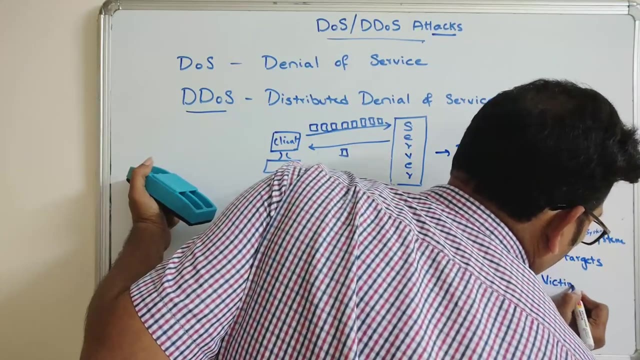 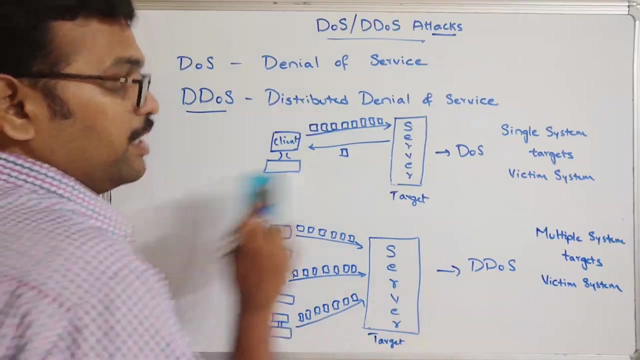 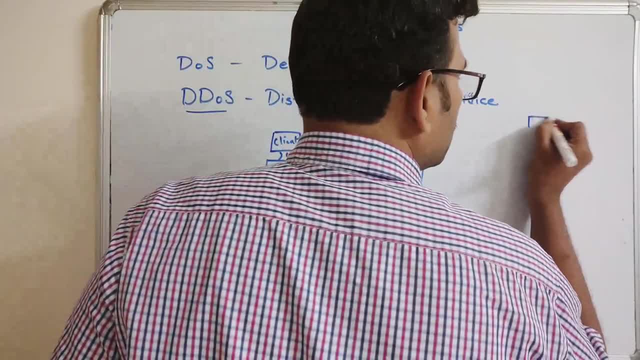 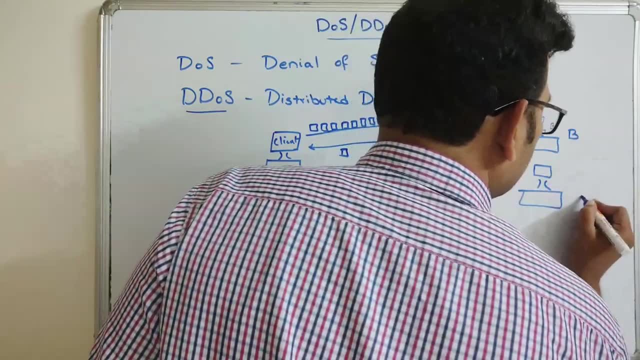 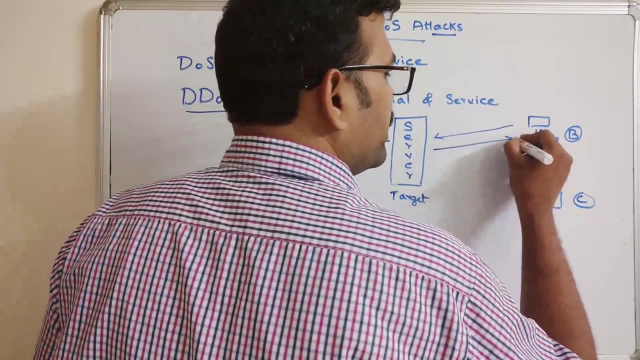 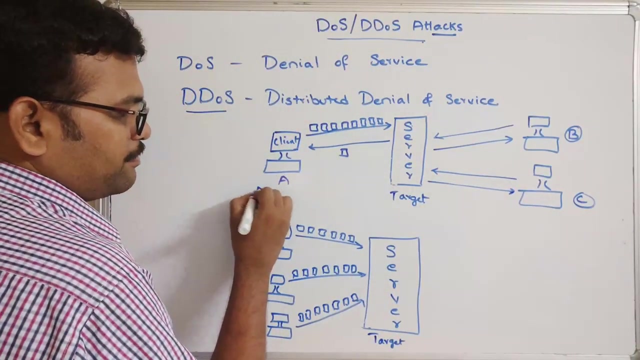 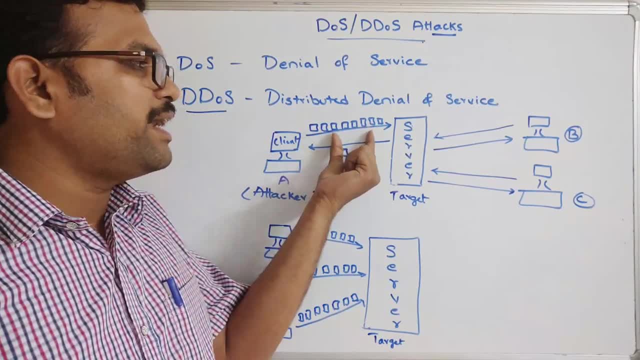 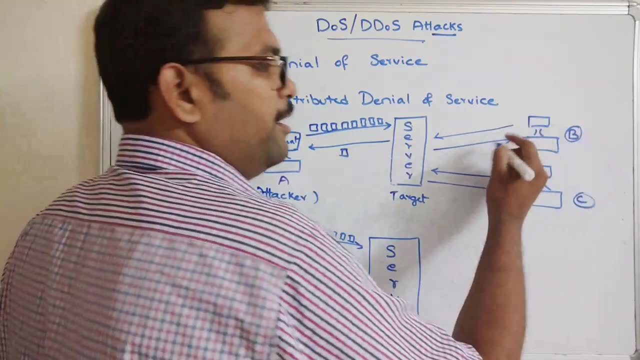 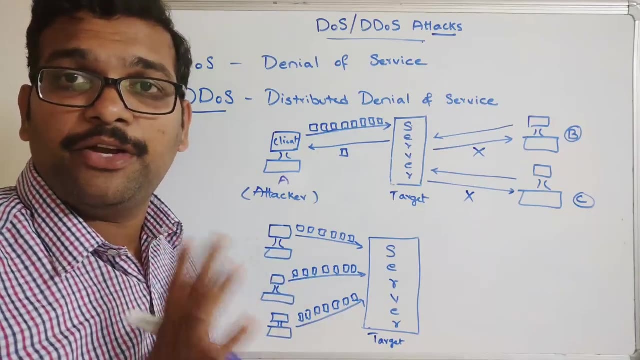 continuously flooding the target with the traffic. that means sending more number of requests automatically. the server will not respond to A or B or C. So B and C are the genuine. that means the legitimate users, but still they are not able to get the service from the server. 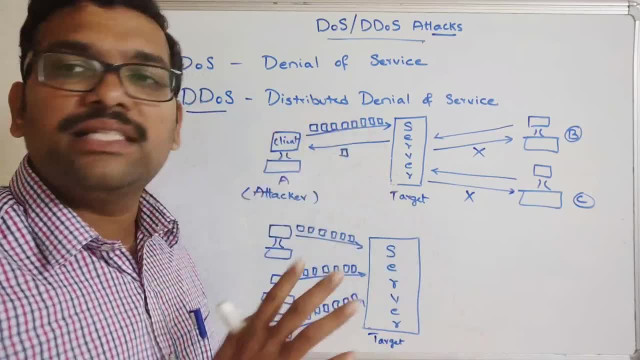 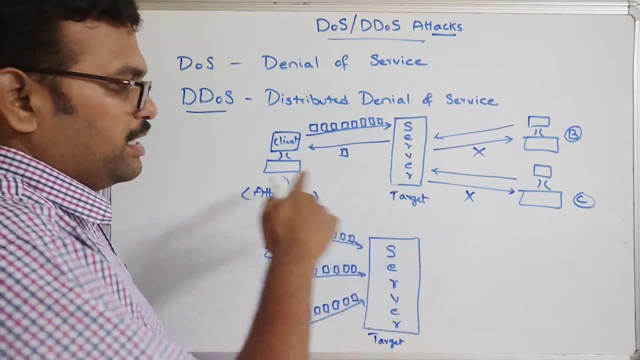 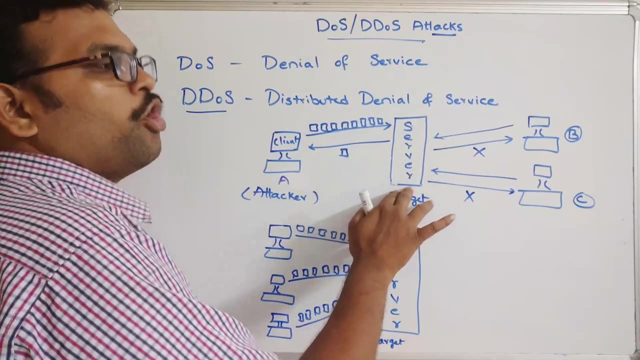 So that means they will think that the server is refusing the response. So such type of attacks we call it as a denial. That means this client, that means the attacker will make the server down and it will make not to respond to the remaining clients, the legitimate users. 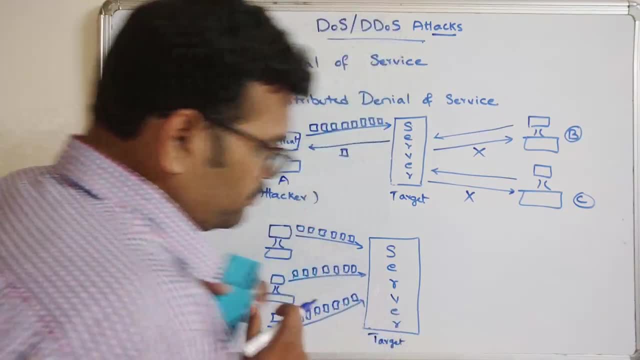 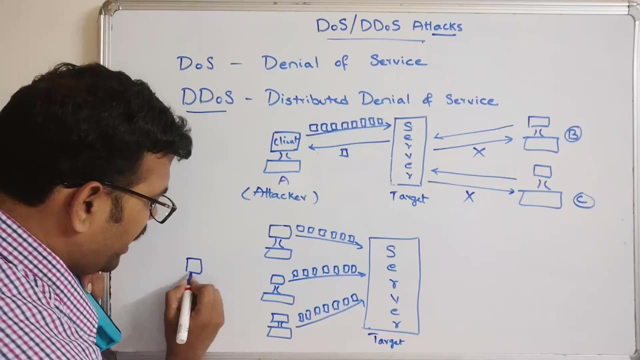 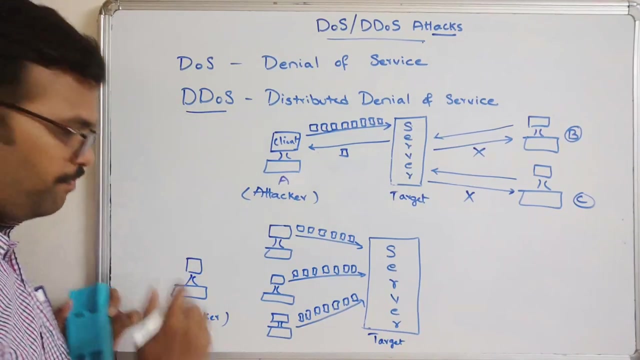 Here also the same thing. So here, multiple systems, multiple systems, So actually. so one system will be there. It's an attacker system, So the attacker system will find the vulnerabilities. For example, this is a A and this is a B. 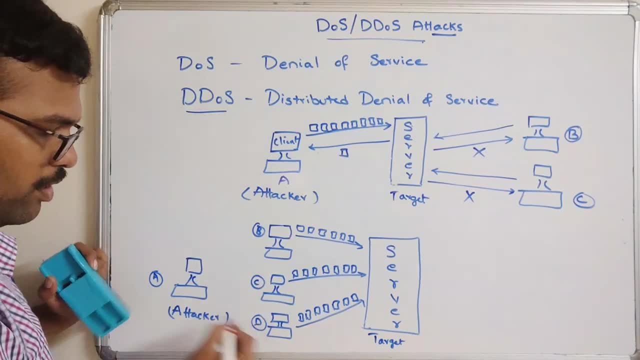 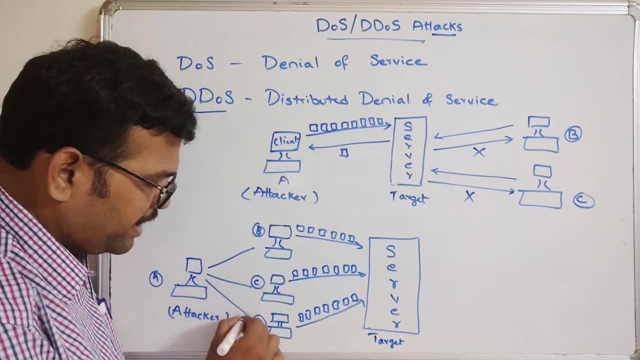 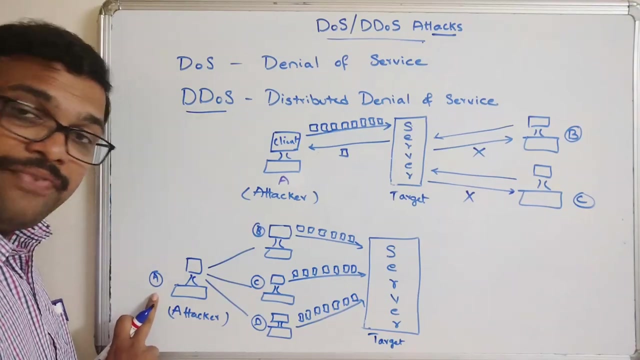 This is a C and this is a D. So once the attacker take the control of one system, the attacker will send the malware to the remaining systems of the network. It will infect the other systems. So once A got infected and the A is the attacker, and that system will send a malware and 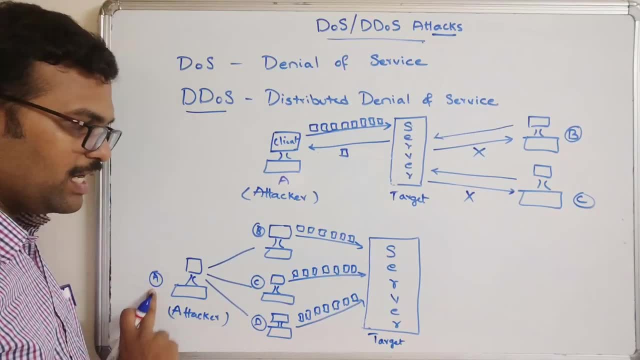 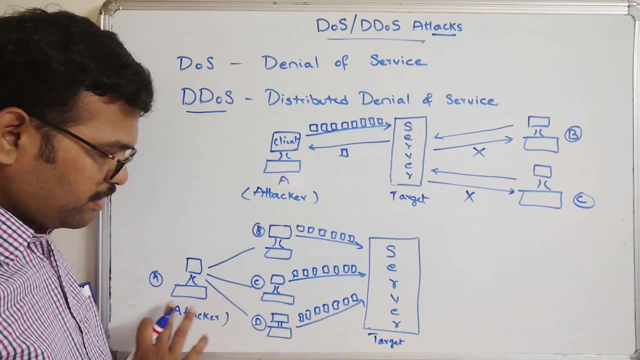 gets the control of other systems of the network. That means A gets the control of B, A gets the control of C, A gets the control of D by sending the malware Right. So once A got the control of all the other systems, 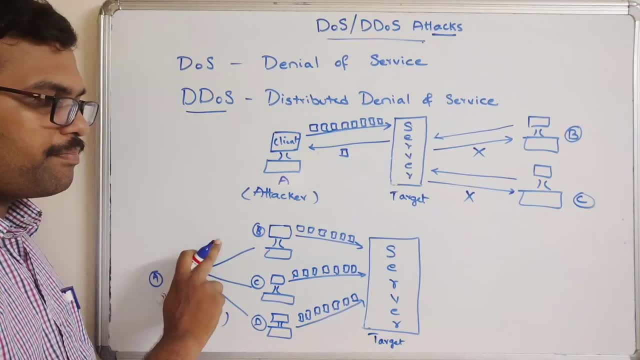 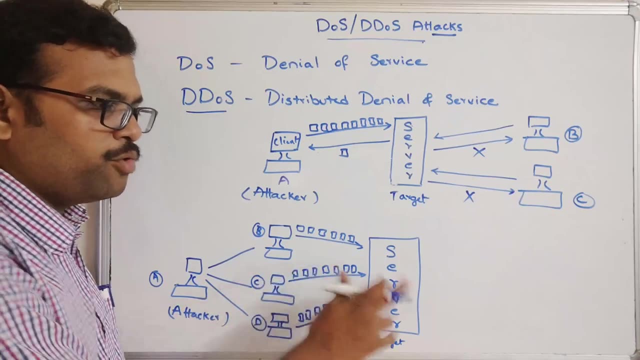 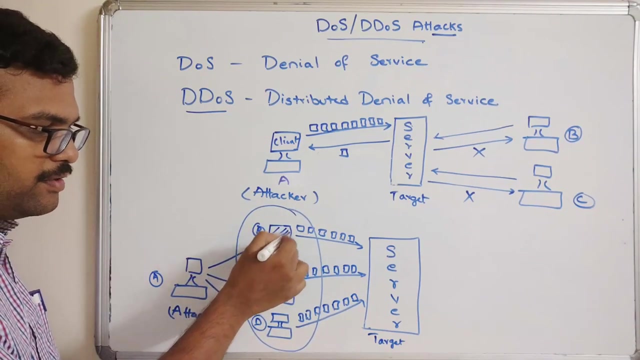 so A will make sure that the complete request, a flood of requests, should be sent by B, C, D at a time to the server. And this type of network, that means a network with the infected, a network with infected, so this is an infected system, right. 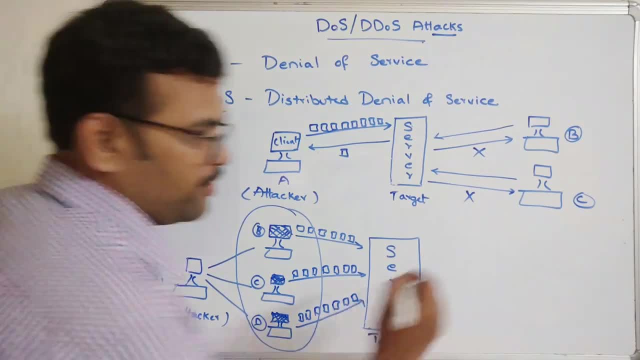 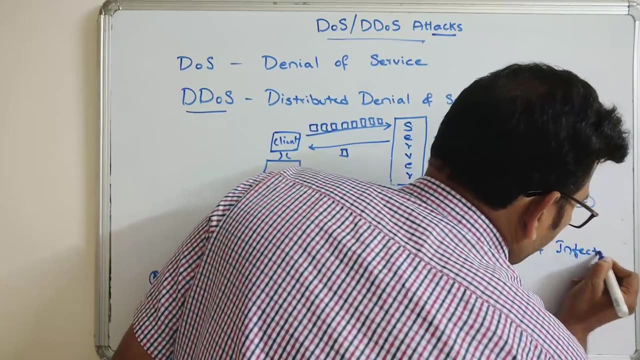 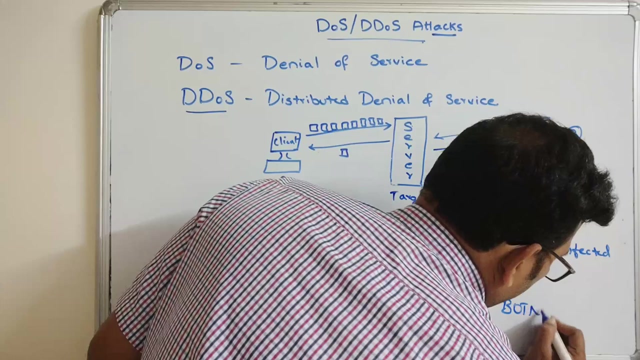 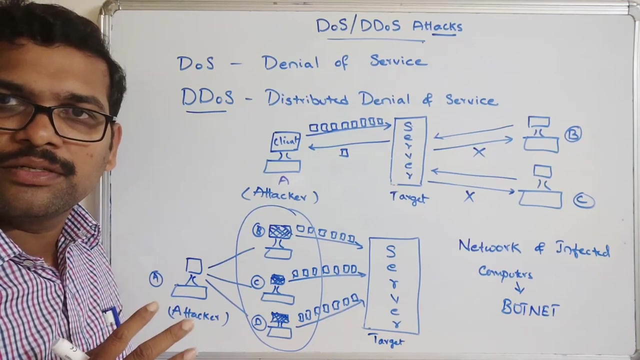 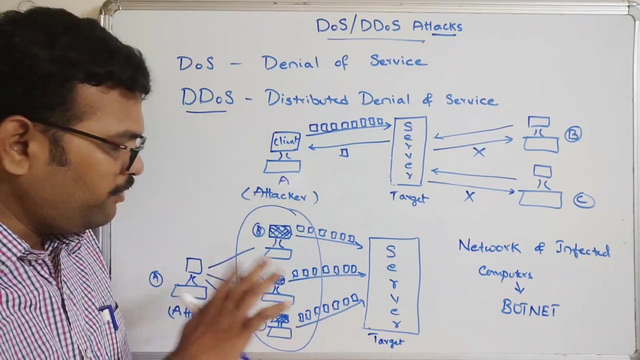 So infected systems is called a botnet. okay, a network of infected computers, infected computers is called botnet, And each system we call it as a bot, Each system we call it as a bot and that will infect other systems. Obviously, now it is three and these three systems will. 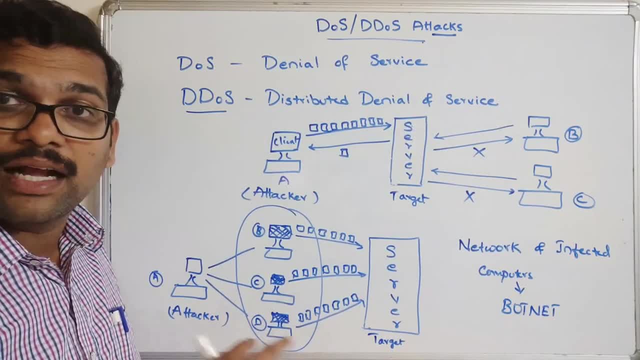 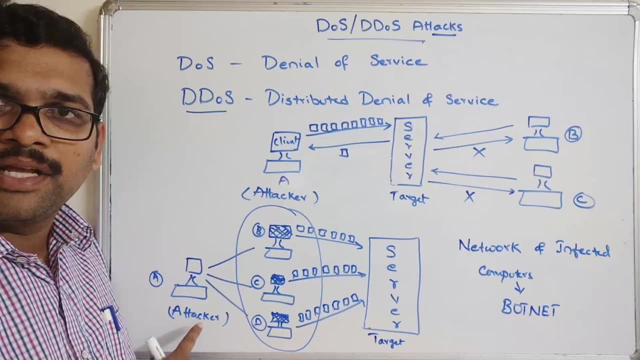 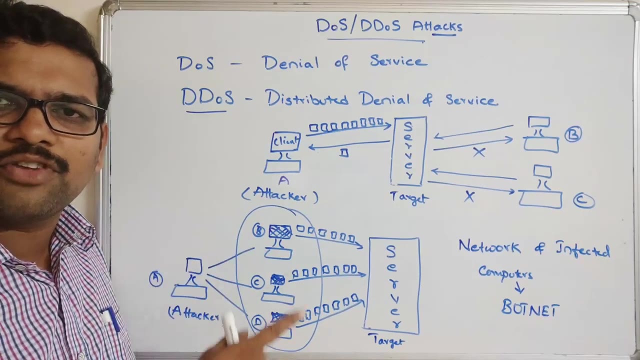 also infect other systems. So, like that, the complete network, the systems which are available in complete network, will be under the control of attacker. So at a single time the attacker will trigger an event so that all the systems in the system, I mean all the systems of a 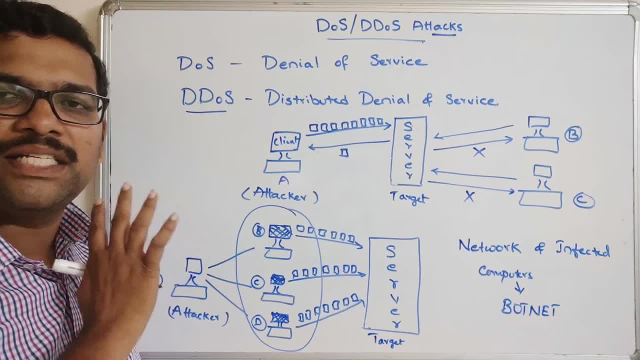 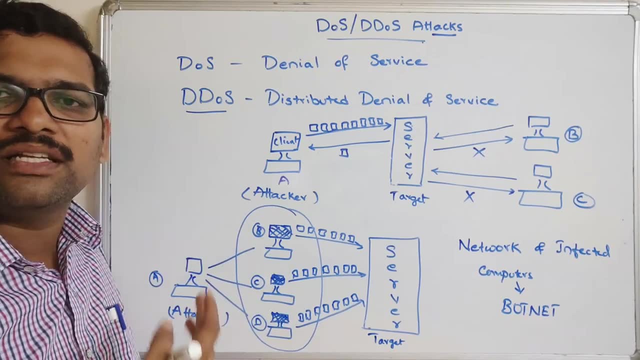 network which are infected will start sending the messages or a request to the server. So obviously the server will receive a lot of requests. So obviously the server can't respond to all the requests Automatically. the server will be getting down and it.